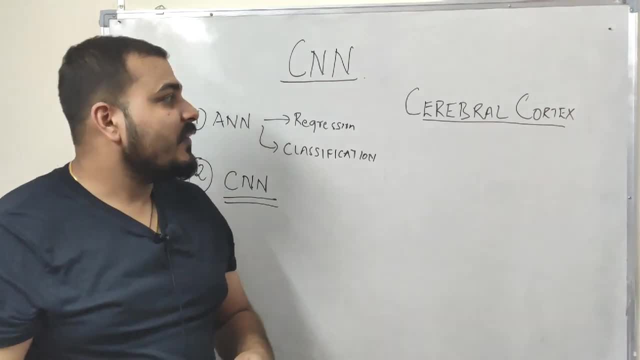 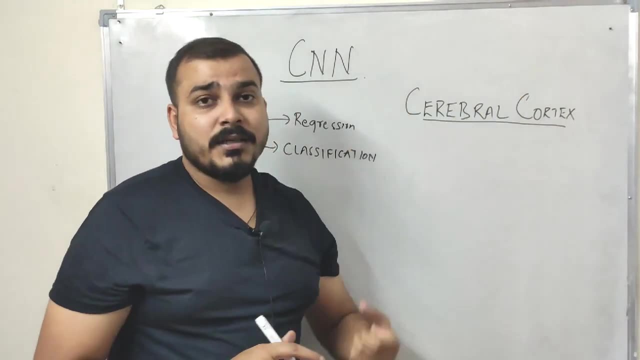 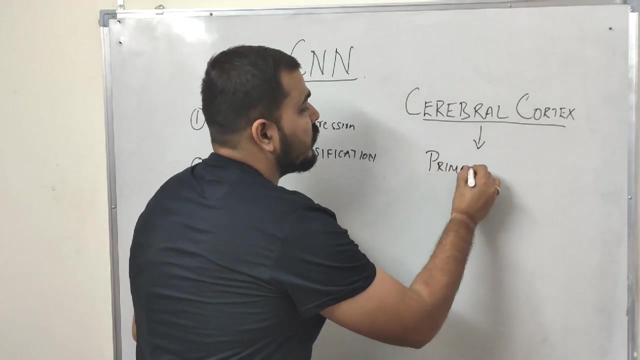 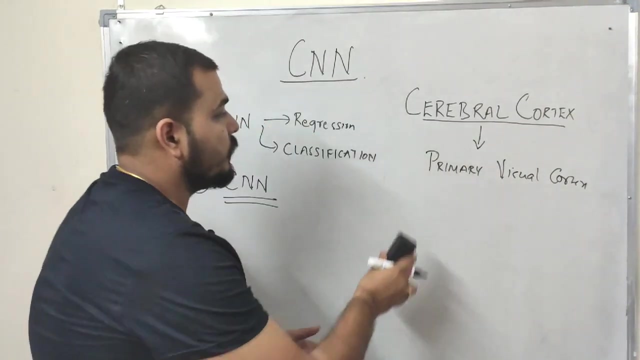 head right over here. in this particular region we basically have something called a cerebral cortex, and you know that human brain is basically divided into four parts and one of the parts is basically called as cerebral cortex. inside this you have something called as primary visual cortex. sorry, should not be primary, it is just visual cortex. so 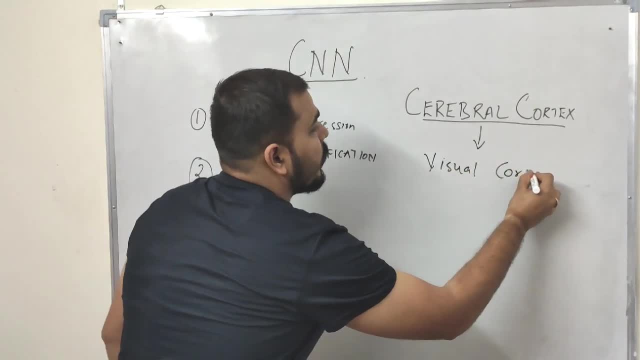 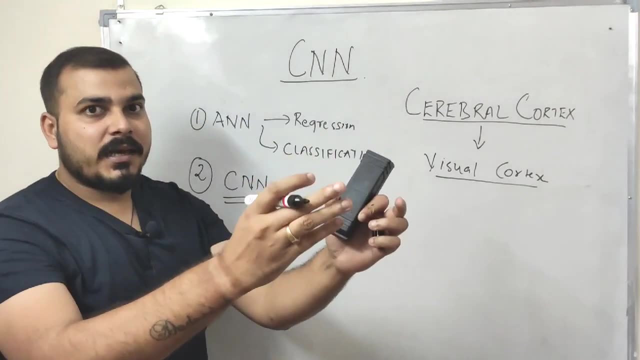 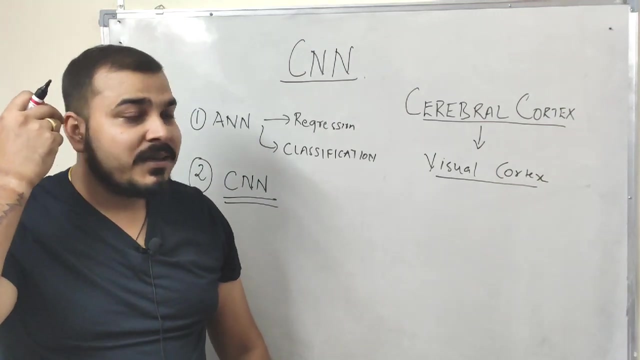 you basically have something called as visual cortex, which is basically responsible for seeing the images. so remember, guys- suppose I am seeing a cat. right, that information passes through my sensory organs, that is, eyes. once it passes, it passes through various neurons and then it reaches this particular region where there is something called as visual cortex, in visual cortex also. 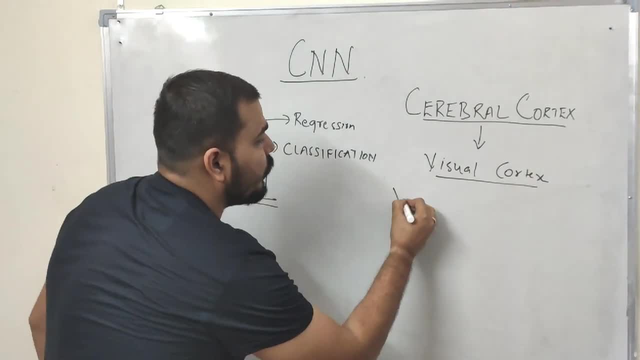 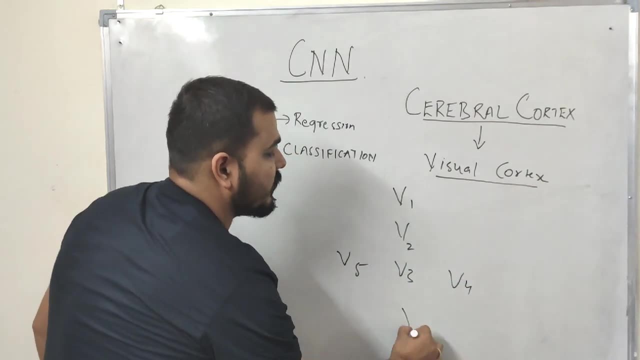 you have multiple layers, okay. you have layers like v1, you have layers like v2, v3, v4, v5 and v6. I've just defined in this way. so what will happen is that this layers play a very, very important role in the visual cortex. so what will happen is that this layers play a very, very 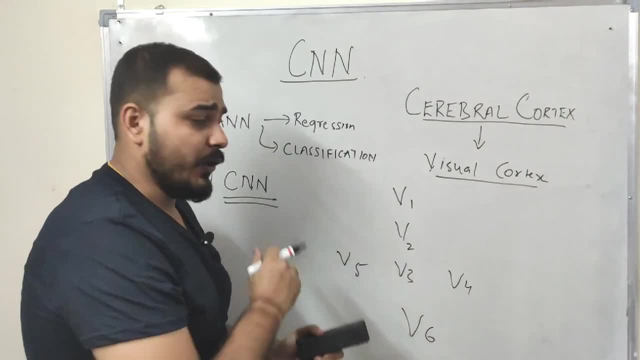 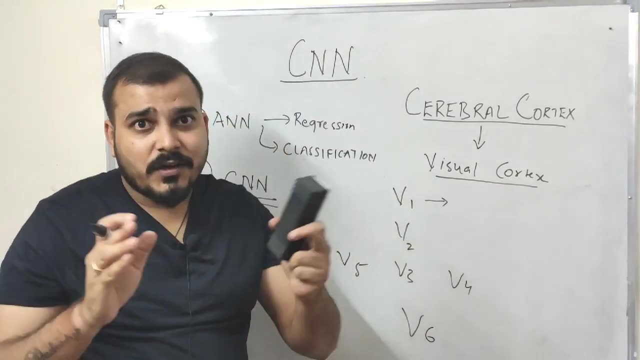 important role. now how it plays a very important role. I will just try to explain you now. suppose, consider that v1 layer is basically responsible for finding the edges of that particular image. now let me see, suppose I'm seeing a cat. I want to find out the edges of the cat. 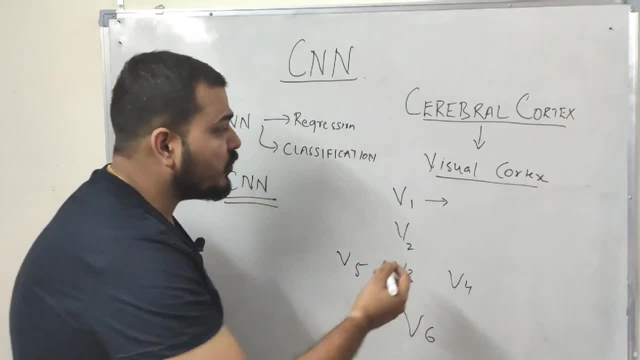 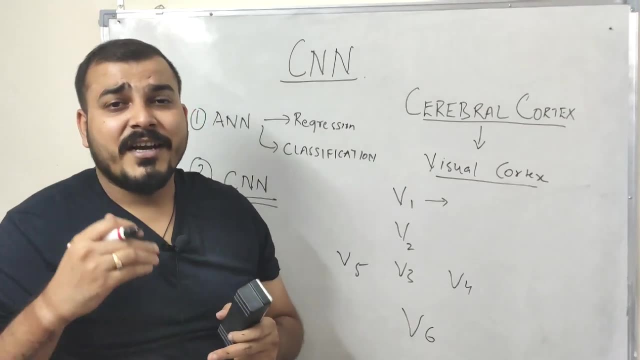 like his ear, edges, his eyes and all. so those, all information will be passed- will be mostly calculated by this v1 layer. I'm just taking as an example. it may not be precise, but I'm trying to say you that this layer will be be responsible for determining some information from that images. okay, and 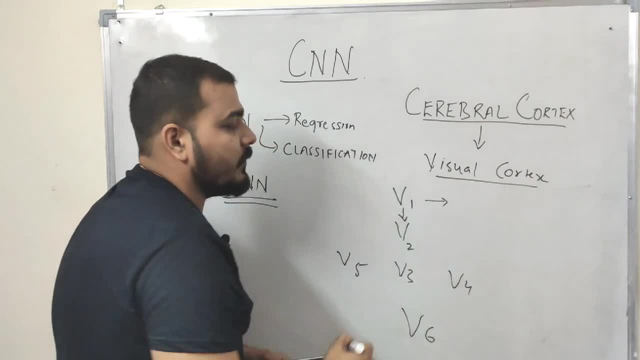 after that it passes right. then it goes to the next layer, it goes to the v2 layer. now this information, what we have passed to the v2 layer- some more information will be done- will be gathered from this layer also. so that basically means that it will try to determine whether the object is moving. 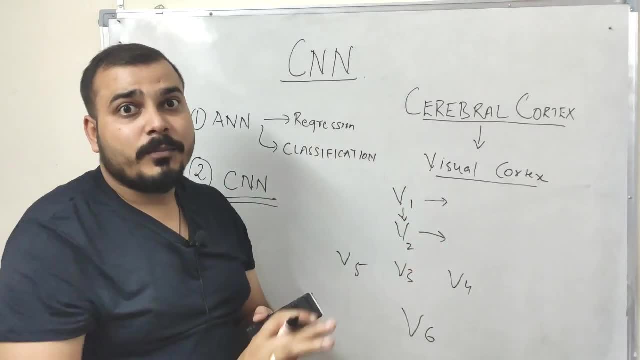 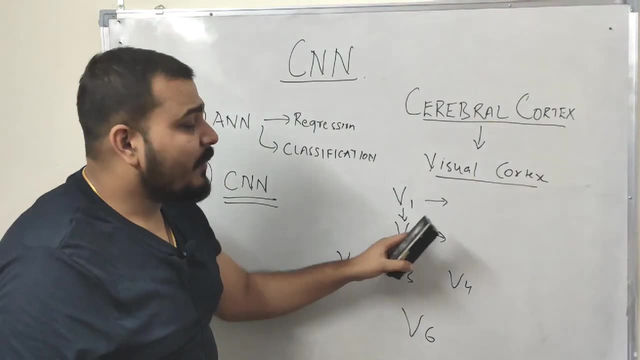 okay, and apart from that object, is there any other object along with that? suppose there is a cat and a dog, if there are two objects, is it able to determine that two particular objects? so multiple objects can be determined. again, I'm saying you guys, these are just examples what I'm telling you, but the main thing, 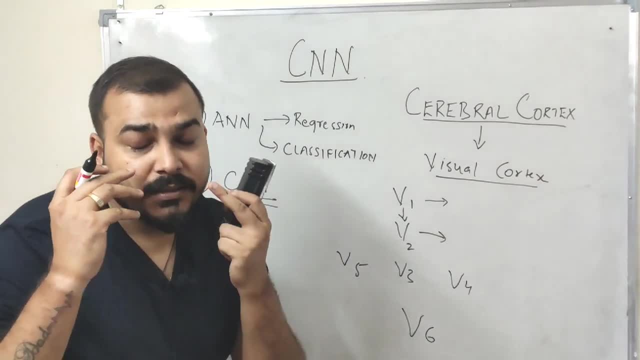 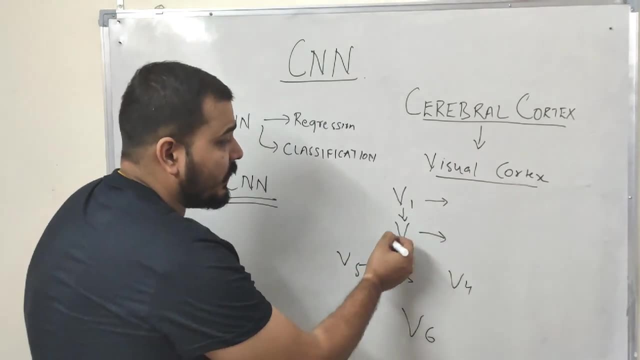 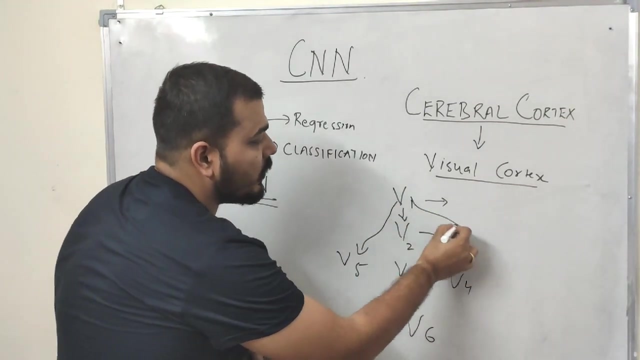 that you need to understand is that each and every layer does some, does some kind of operation where you are extracting some information from that images or from that video frames, okay, and finally you'll be seeing that after, suppose, in v2 layer, something happens right. similarly from v1 to v4, v5, this all 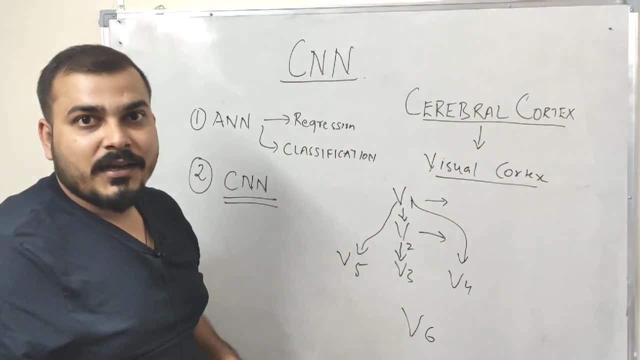 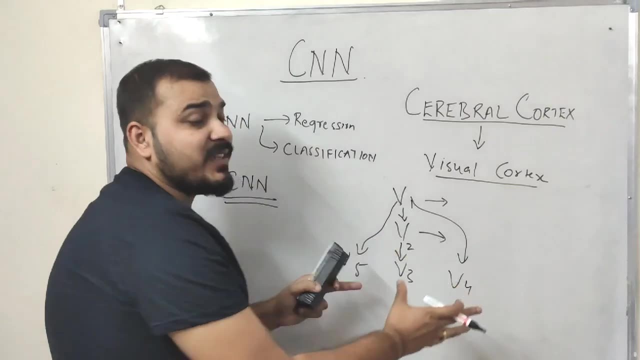 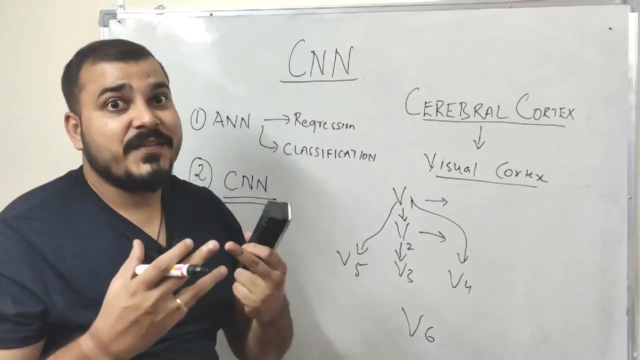 information also gets passed v2 to v3, right. so when this information is getting passed, each and every layer will be responsible for doing some other kind of operations. now, what are the specific operations that I'll just discuss when we will be discussing about CNN in my next class. where, specifically, 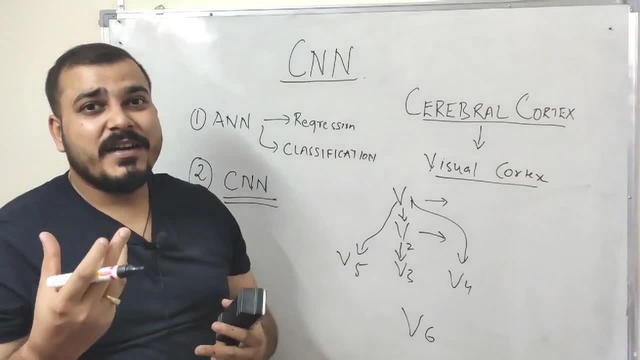 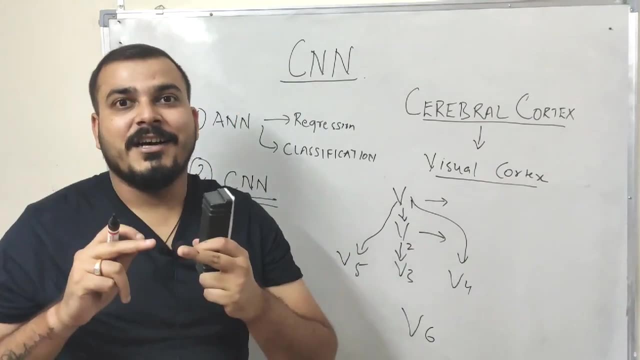 in CNN you call it as filters. okay, now, each and every filter is responsible for. suppose one filter is responsible for finding the edges, one response, one filter may be responsible for finding the face shape, so all those kind of stuff over here. v4 layer is specifically used for 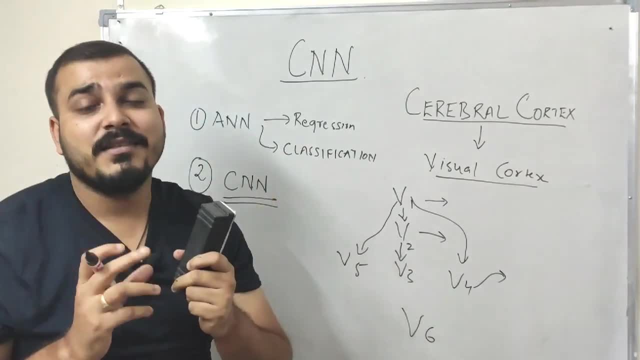 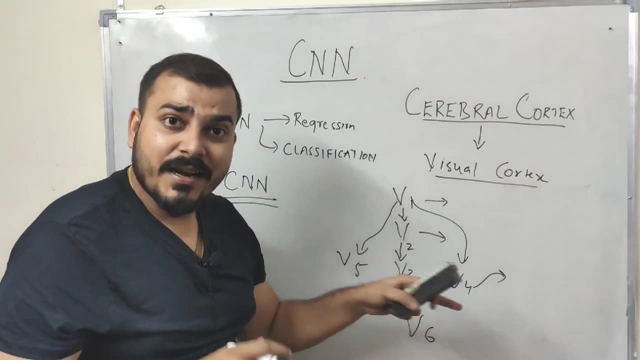 seeing the edges of the object. and then, when you see the edges of the object, you see some layers and then you can define the base layer that you want. ie, this was here. and then, when you see the edges, here is where the boundary layer will bin, nurture the inches, and here, a Teka layer is where the bara will be. 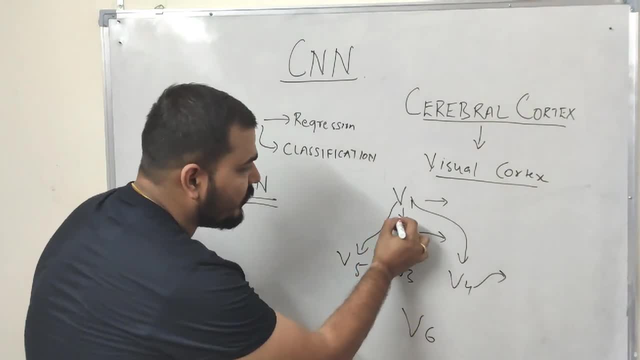 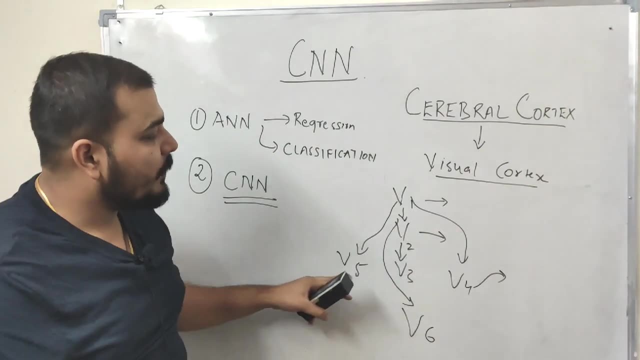 attached to the edges and this 서울 or this one is formof a Saul wheezer do, which is going to give some effect on the edges and also from inside of thefishes. okay, you can do some controls also too, like if you zoom up you can see all that stuff right, and because it's automatically in the section. you'll be getting enough of trust. so it's going to be this. and if i drop this one here and then if i grab it and my look like this and i wait something like this, that look like this, so this stuff actually. 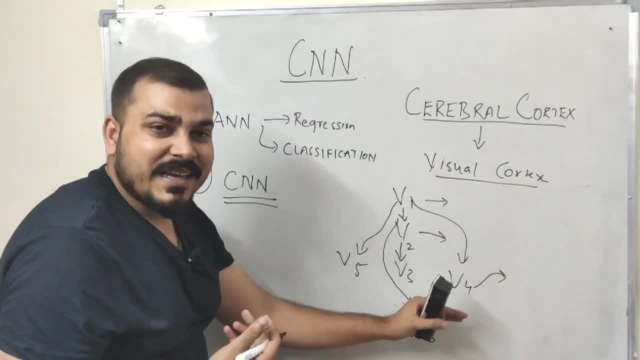 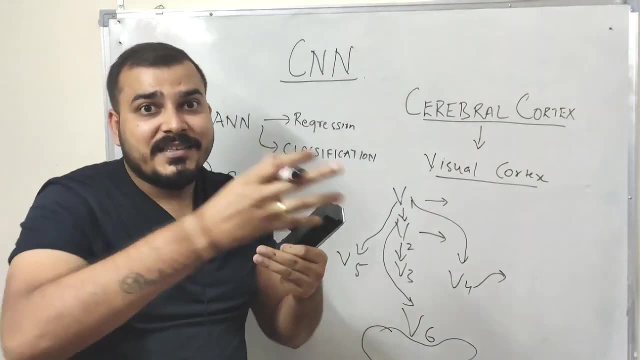 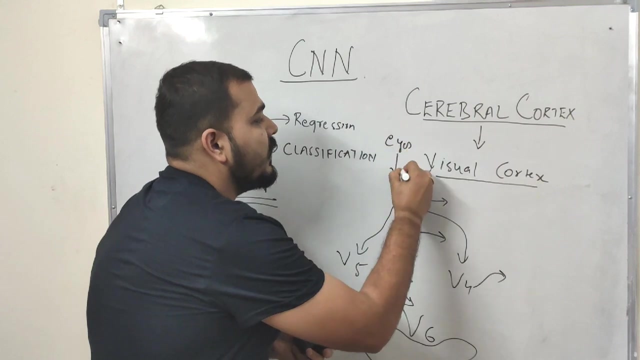 some of the information. okay, now, once all this thing is done, finally, our image gets, you know, imagined away. it gets created over here and hence we are able to visualize and say that, okay, this is a cat, this is the dog. but just understand that as soon as the information is passed from our eyes, right and this, 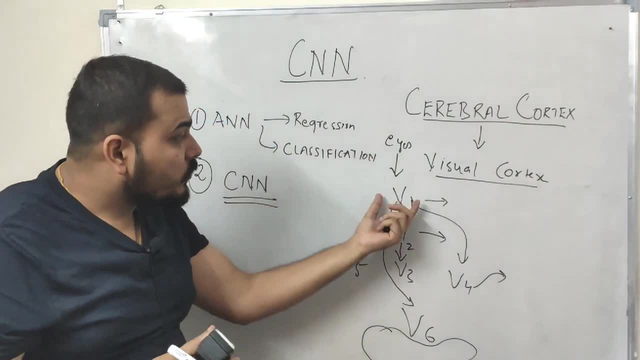 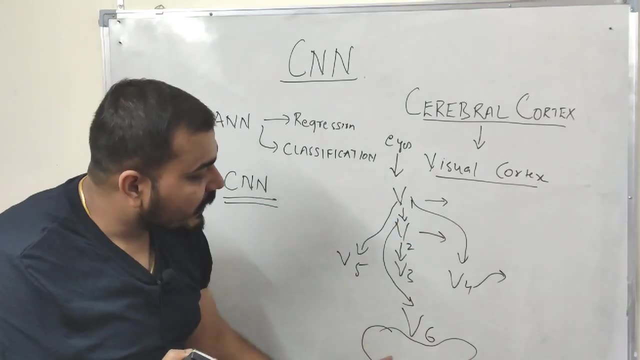 particular information is getting passed through our sensory organs and then it will pass through all this particular layers where there are little little bit bit of information that is getting extracted and finally we are basically able to see that because it is basically getting created over here. I'm.